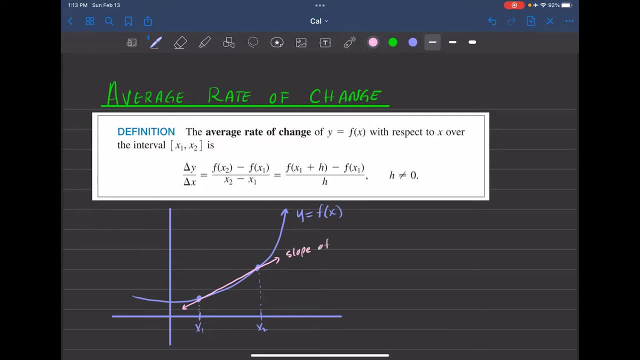 the slope of this secant line is what we call the average rate of change. Well now, how do we find slope? Well, as you remember from algebra, slope is pretty much changing y over changing x. So we look at the change in the y value. So think of it as this is the rise. 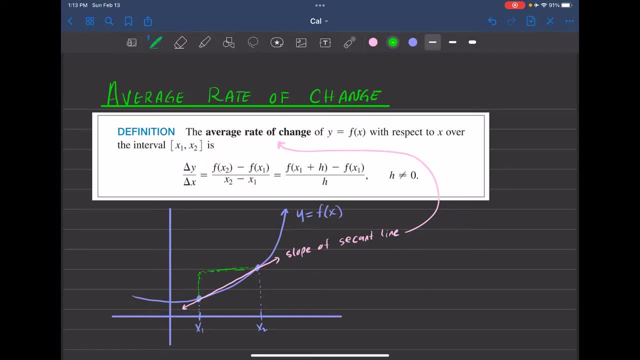 and then run. So we create this triangle And find the change in the y value over the change in the x value. So that's what we have right here, Or you can think of it as this is the rise over run formula from algebra. 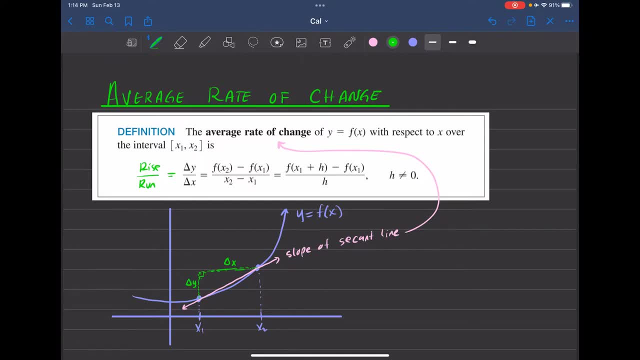 So the way you're going to find that change is so we know the first point was x1. That means this point right here is the function evaluated at x1. So that's f of x1. Then the y value of the second point right here would be f of x2. So that's where we have f of x2 minus f of x1 divided by. 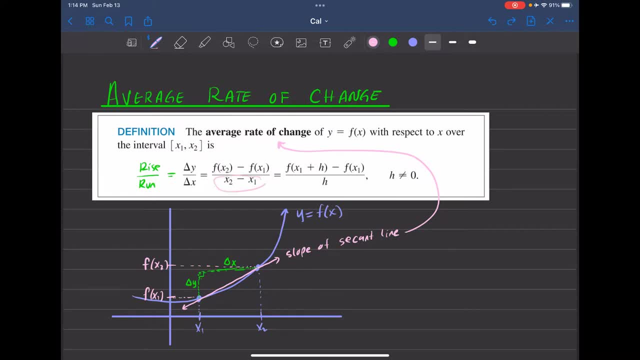 the change in the x direction. That's x2 minus x1.. Now, later on in the future, we like to simplify the notation, So instead of calling x2, we're actually going to call this point just a little bit more than x1.. So let's say x1 plus h, Which means 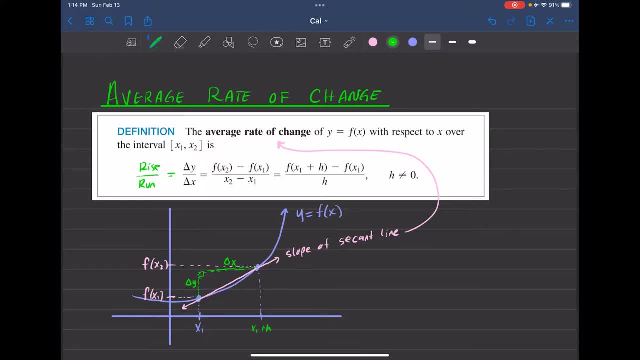 so we're actually going to call this point just a little bit more than x1.. So let's say x1 plus h. So let's say x1 plus h, the second y-coordinate. I can also write this as f of x1 plus h. And then we get to this formula. 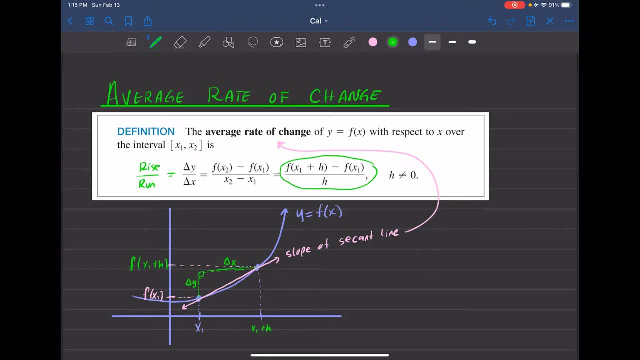 right here. Now hold on to this dot until we get to the tangent line idea, because that's when the notation will be much simpler to use. We would rather use this one versus this one. So now that we have a little understanding of this formula, let's go ahead and try to do some examples. 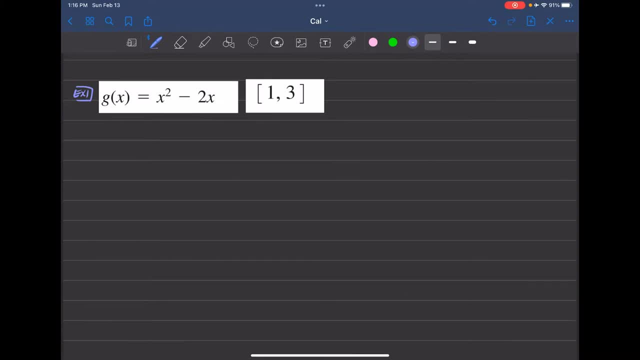 So here's our function, and we want to find the average rate of change within this interval. So let's go ahead and do that. So we know that the average rate of change is given by f of x2 minus f of x1, over x2 minus x1.. You might have known this formula in a different form. 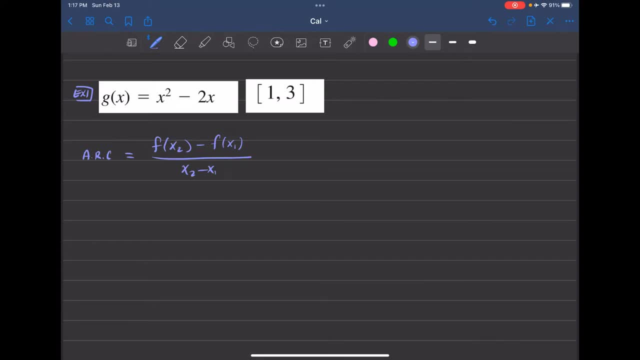 but this is the one I'm going to use it here. You might also have known it as f of b minus f of a over b minus a. So this is also the same formula for average rate of change, Instead of x1, x2,. 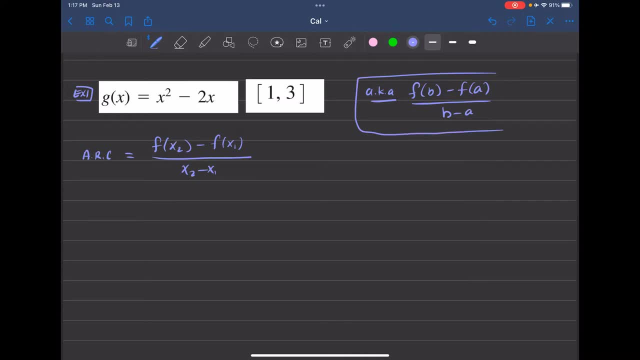 we're using a and b, So it simplifies a little bit more, But let's use this one, since that's the one I introduced previously, But feel free to use the one on the right if you feel comfortable. So let's go ahead, and. 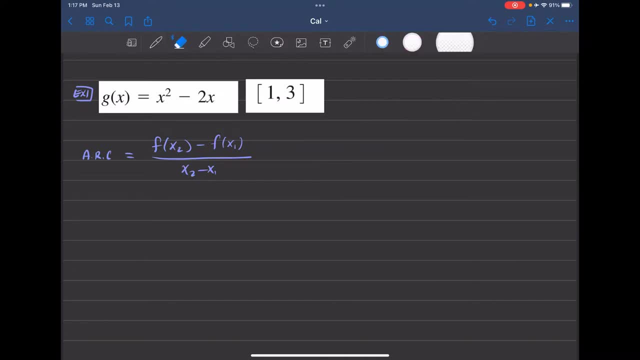 label our x1 and x2.. The first coordinate will be the x1.. The second one will be x2.. So we need to find f of x1. So f of x1 would be f of 1.. Plug in 1 into the function. 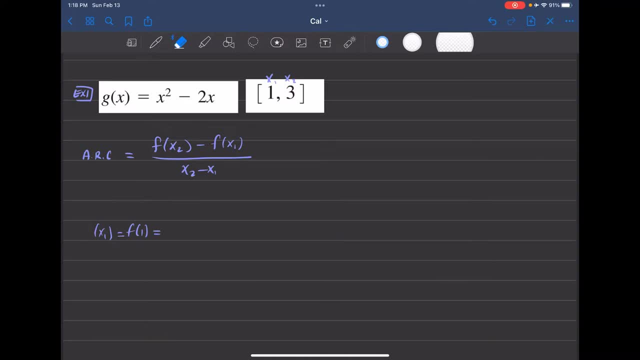 Now in this notation we're going to be using g instead of f, Just switch a little bit. So g of 1 is going to be 1 squared minus 2 times 1.. So that's 1 minus 2. That is negative 1.. And then g of x2 is going to be g of 3.. 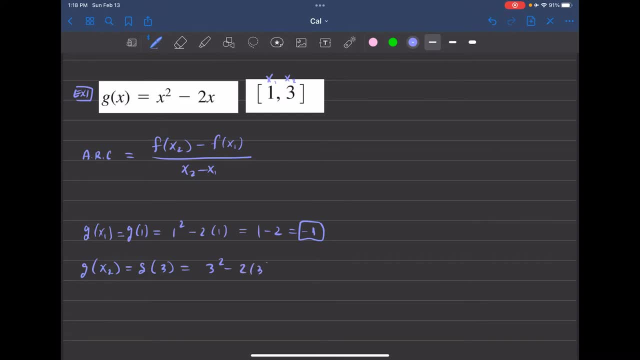 That is 3 squared minus 2 times 3.. That would be 9 minus 6,, which is 3.. So we found our function values. Now let's simply plug this into our formula right here. So we're looking at g of x2. 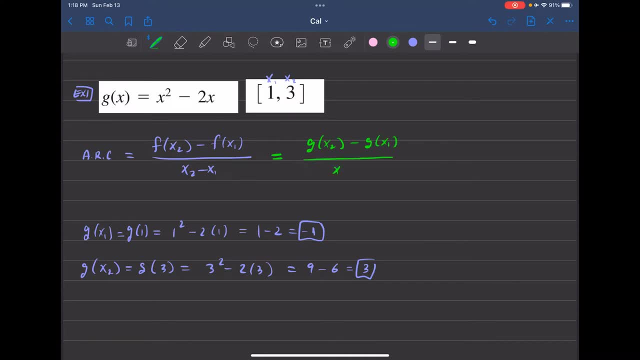 minus g of x1. So we're going to be using g of x2 minus 2 times 3. That would be 9 minus 6, which is 3.. 1 divided by x2 minus x1. So in this problem, this is our g of x2.. This is our g of x1. And x1 and x2. 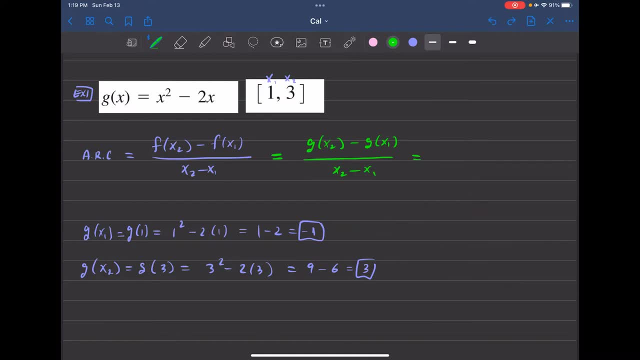 are these points right here? So let's substitute them. So we have 3 minus negative 1, because that's g of x1, over x2.. That is 3 minus 1, which will give us 4 on top over. 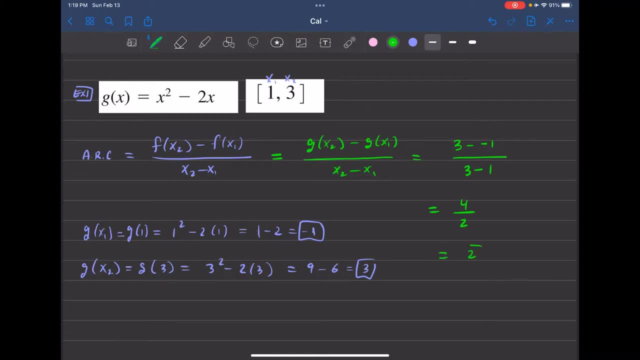 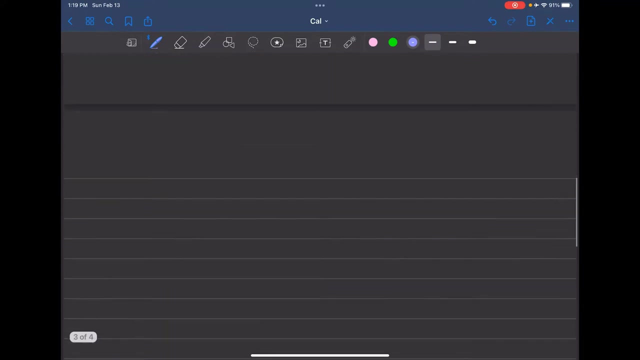 2 on the bottom And that simplifies to 2.. So the average rate of change or the slope of the secant line on this interval happens to be 2.. All right, So let's go ahead and try another example. So let's say we want to use the function. So this is our example 2.. f of x is equal to 1. 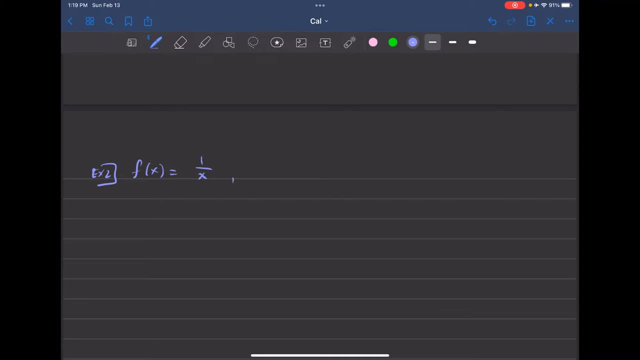 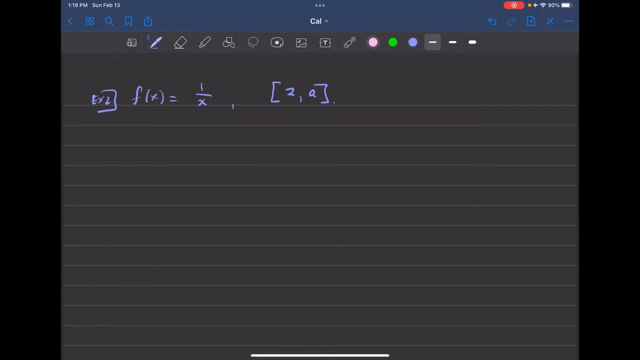 over x And we want to find the average rate of change on the interval 2 and some a. It could be any real number. We just want to try out with some arbitrary real number, a. So we'll do the same thing Again. if you want to try it out on your own, pause the video. 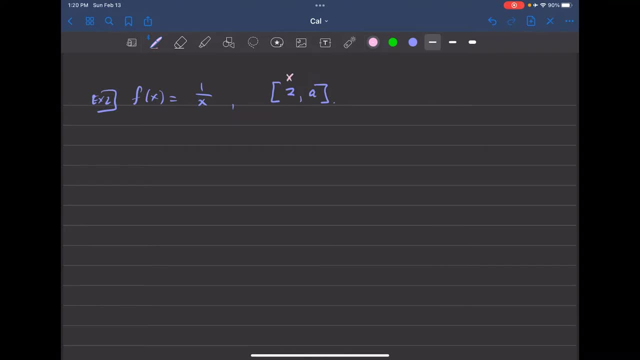 work it out and then come back check again. Let's call this 1x1, this 1x2.. We want to find f of x1. That's going to be f of 2.. Plug in 2 into the function. We get 1 over 2.. 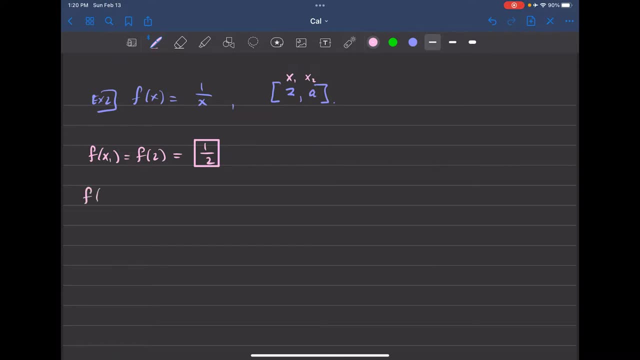 So that is our f of x1.. Now for f of x2, we're finding f of some a. Again, we replace a where there is x in the function. This is simply 1 over a, And that doesn't simplify, so we leave it here. 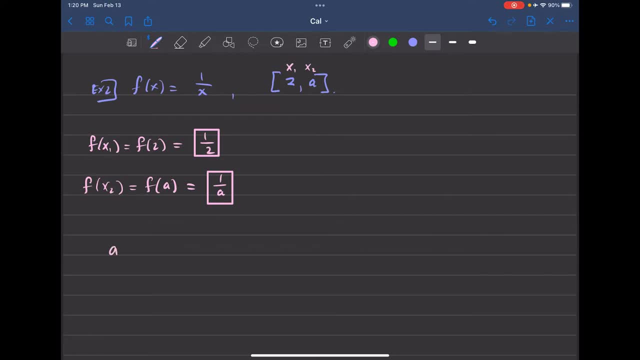 Now we're ready to find our average rate of change. So the average rate of change over this interval would be f of x2 minus f of x1, over x2 minus x1, which would be f of a minus f of 2, all over a minus 2.. 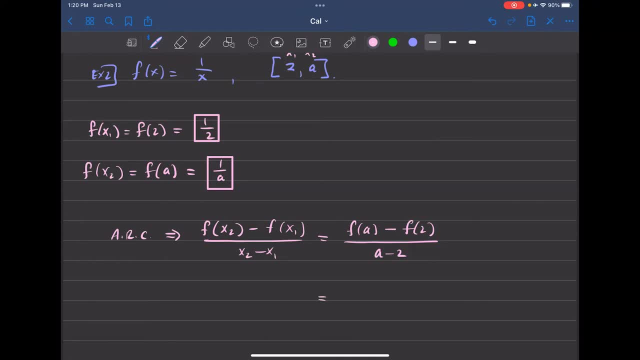 And then we plug in what our function values are. For f of n, it is 1 over a minus f of 2. That's 1 over 2, all over a minus 2.. Now you want to simplify this a little bit more, because we have fractions right here. 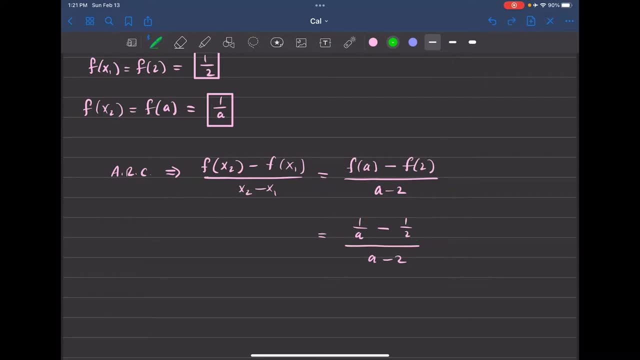 We want to combine that, the least common denominator, to combine that. So the least common denominator for the two fractions on top is 2 times a. You need this and that. So now we multiply each fraction What they're missing to obtain the common denominators. So I multiply this with 2 over 2, this with a over a and that. 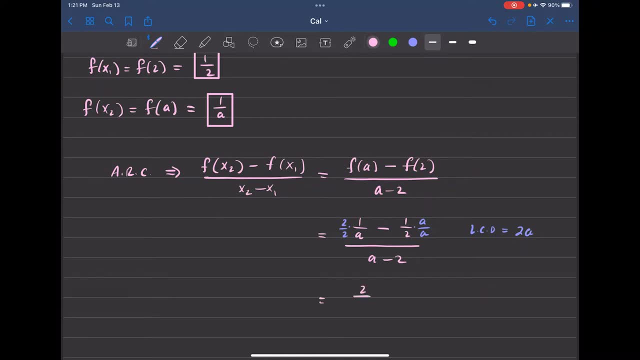 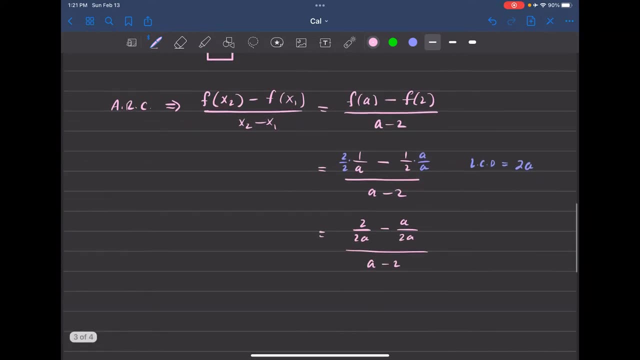 gives me the following. So on top I get 2 over 2a minus a over 2a, all over a minus 2.. And now that the top has same denominator, I can join them into a single fraction, That is 2 minus a over 2a. 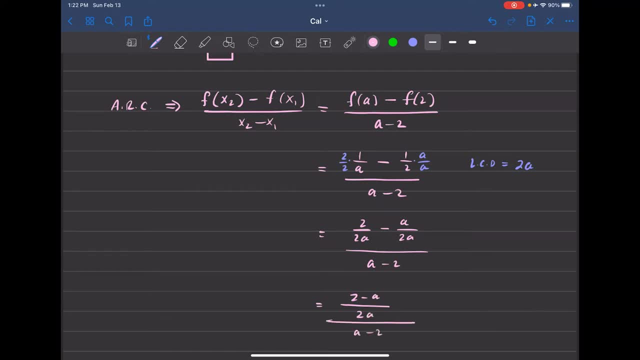 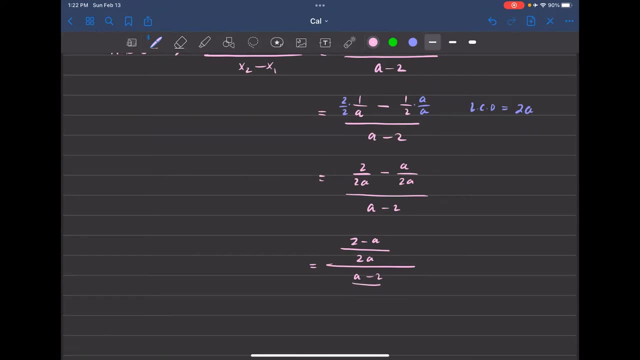 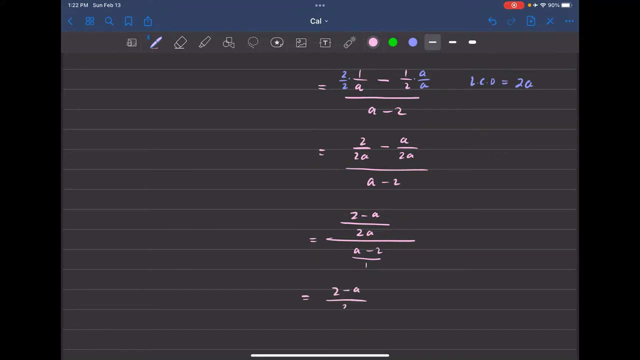 all over a minus 2.. And just continuing on with simplification Now, because we have fraction over a fraction, you can write this as a fraction, like that: 1 over 1.. I can simply write that as 2 minus a over 2a times the reciprocal of the bottom, That's 1. 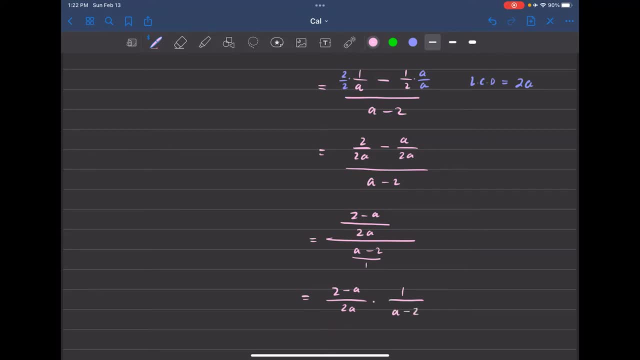 over a minus 2.. Now a minus 2,, if you realize. and 2 minus a. they're almost the same, except they differ by a negative sign. So if I were to cancel them, I must put a negative 1 somewhere to place. 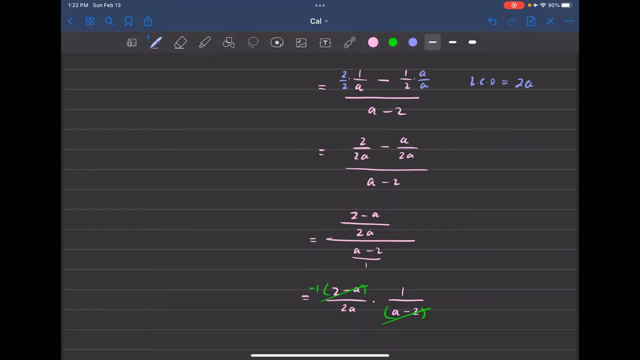 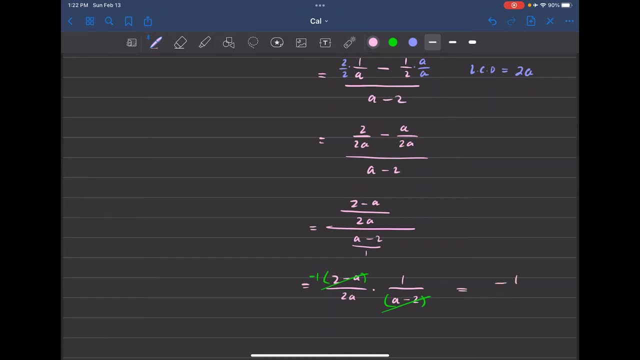 that difference. So in reality, that's what I get by canceling them. I get a negative 1, either on top or bottom, And this gives me negative 1 over 2a as my final average rate of change for this problem. For this problem, we're going to find the average rate of change by using 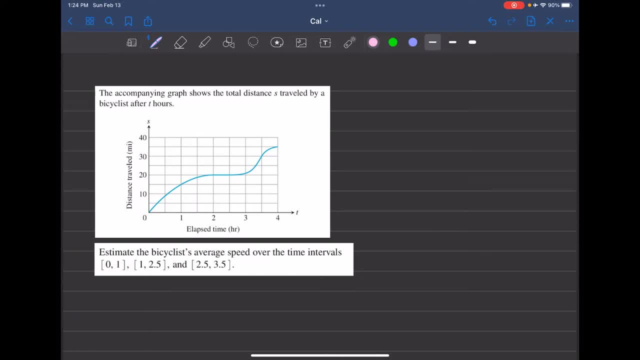 this given graph. So we have this graph of showing the total distance s traveled by a bicyclist after some tea hours. so let's see what we're looking for. we want to estimate the bicyclist average speed, which is same idea as average rate of change. we know that the distance, so the average speed it's the distance traveled. 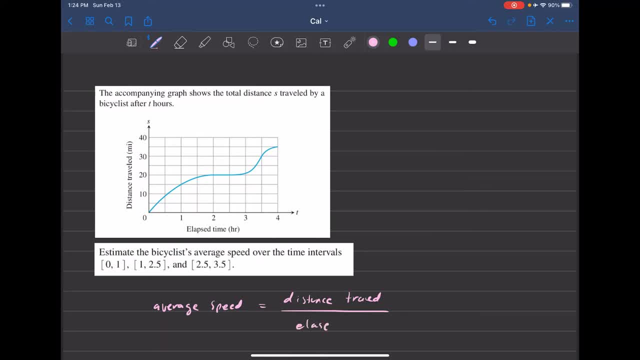 divided by elapsed time, so pretty much the change over Y, change of Y over change of X, just like we saw earlier with those two examples. so we want to find the average speed over this interval zero and one. again, you can call zero, zero, X, one and one is your X two, so the so over the interval zero and one. 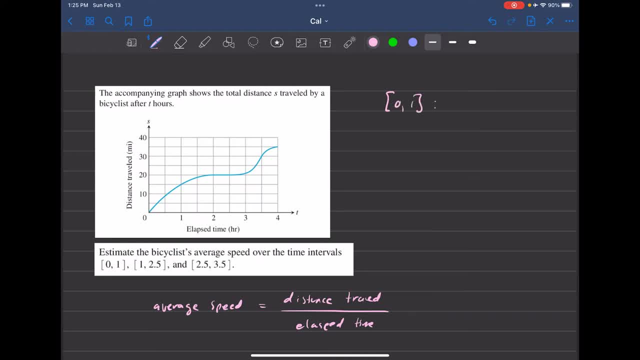 you our average speed. it's going to be, let's call it, average speed. it's going to be the change in distance over time. so I'll be s of 1 minus s of 0, because this is our X 1. this is X 2 over X 2 minus X 1, so that's 1 minus 0. so if you look at, 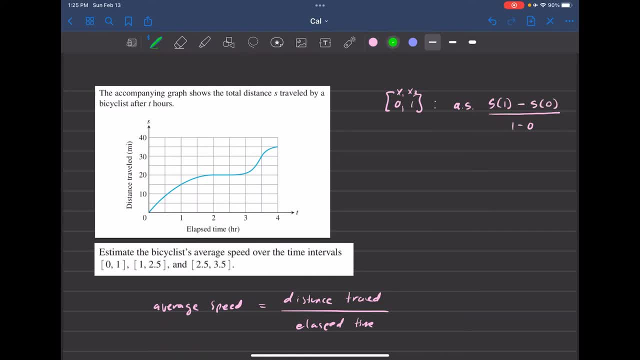 the graph when the time is 1 hour, we're looking here X 2 minus X 1, so that's 1 minus 0. so if you look at the graph when the time is 1 hour, we're looking here and our function happens to be right here. so that's 15, so we can say that s of 1. 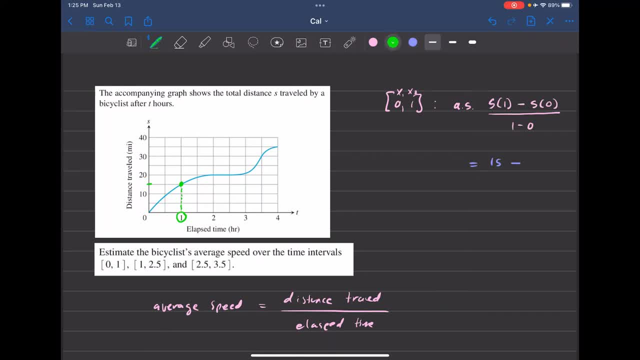 is 15. now for s of 0. we're looking at when time is 0, 1 hour, and the function is right there. so that's also 0. all over 1 minus 0, that's just 1, so this happens to be 15 and we can say this is in miles per hour, so this will be miles per hour. 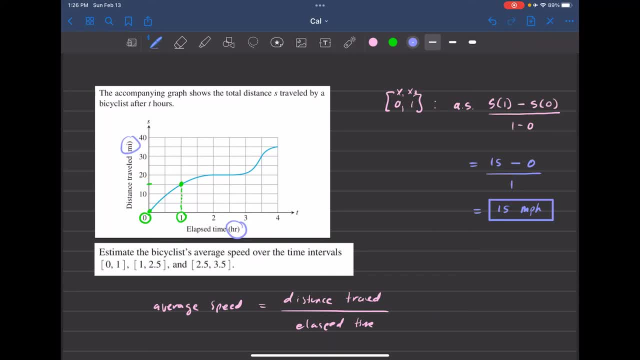 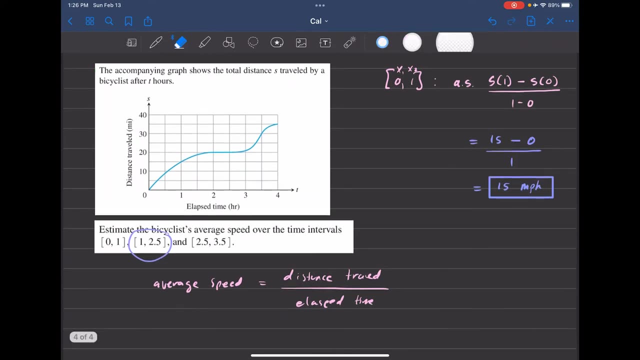 per hour. so the average speed over this interval, 0 to 1, happens to be 15 miles per hour. let's do the same thing for the next part, between 1 and 2.5 hours. so again I will call: 1 is my x1 and 2.5 is x2. so over that interval we have, let's. 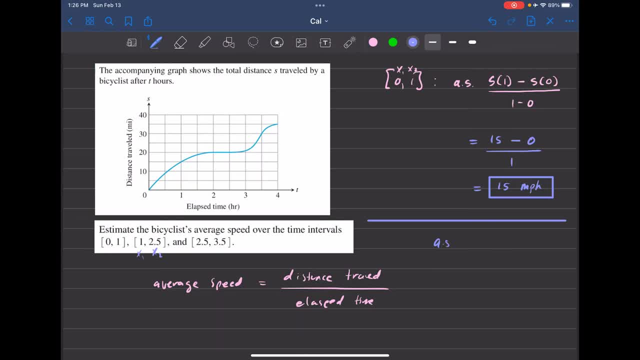 say: um, we're looking for the average speed, which is S of 2.5 minus S of one, over 2.5 minus one, so 2.5 is right here. so the heights we're looking at is this one and that is 20, so it's 20 minus s of one. well, we know what that is, that's. 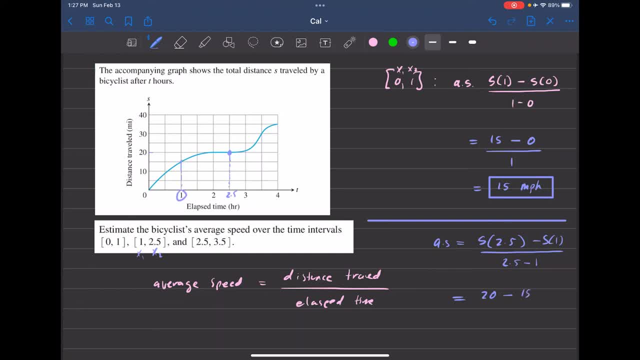 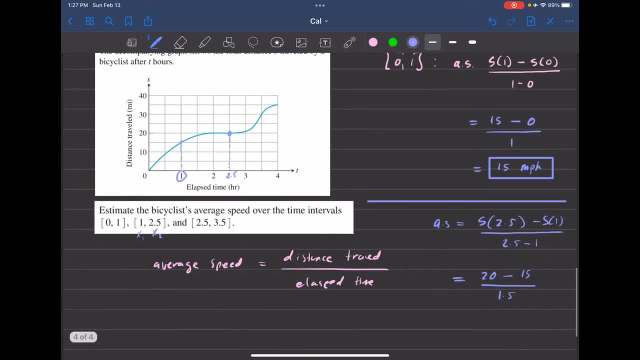 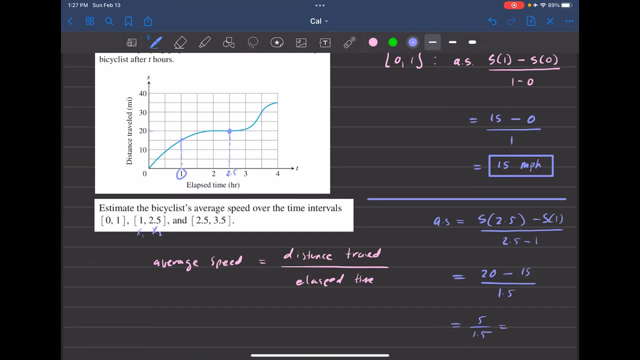 right here and we said that that's 15 all over two point five minus 1, that happens to be 1.5.. So 20 minus 15, that gives us 5 over 1.5, and this is approximately 3.3 miles per hour. So that would be the average speed over that specific interval.